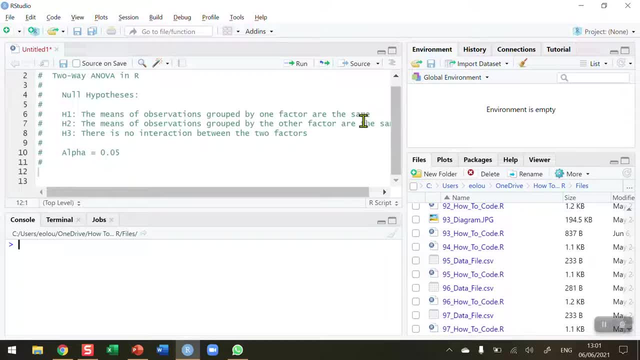 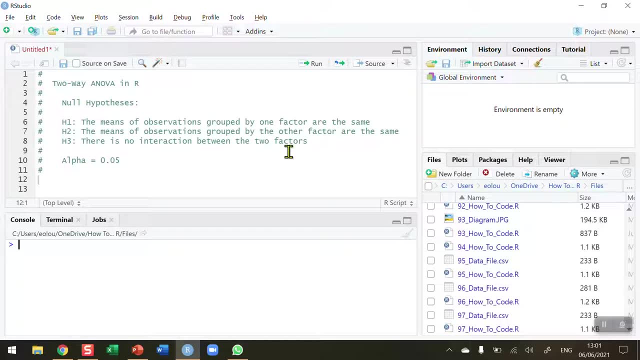 if there's differences between in one factor, so that's hypothesis one. The second factor is tested in hypothesis two. The means of the observations grouped by the other factor are the same. And then quite often the most important thing that we're looking for in a two-way ANOVA. 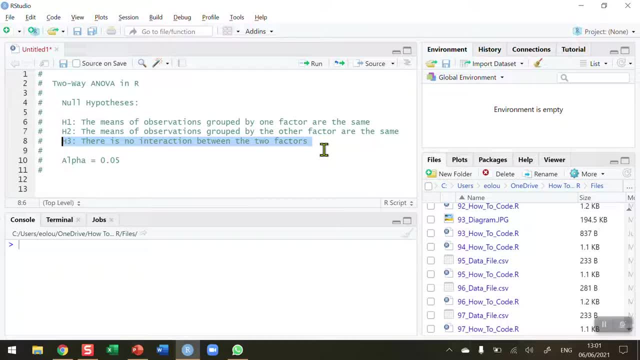 test: is there an interaction between the two factors? So the null hypothesis is that there's no interaction. The alternative would be that there is an interaction. I'm going to call up this test and an alpha value of 0.05.. So the data set I'm going to use in this example is an inbuilt data set in R. It's 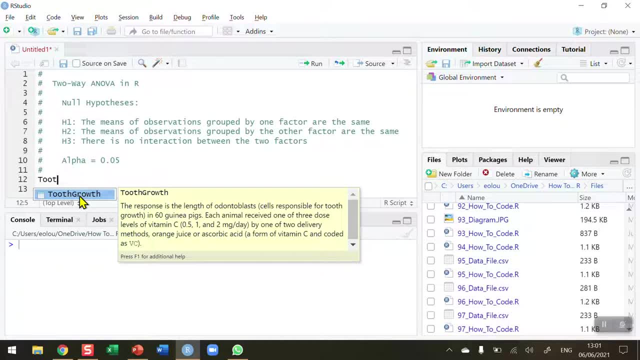 called the tooth growth data set. So we can see here that it is about the 60 guinea pigs are being used and they're being given different levels of vitamin C and also two different methods. So you can look up some information about the tooth growth inbuilt data set. So let's run this line. 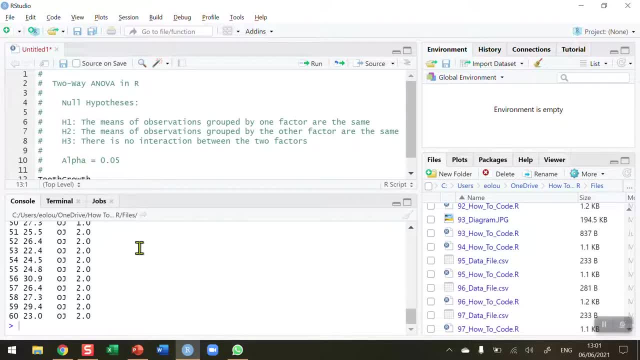 of code and take a look at the data set And we can see when we run it. we've got 60 records, So there are 60 guinea pigs being used here And there's three variables. There's the length in each of the guinea pigs and then there's 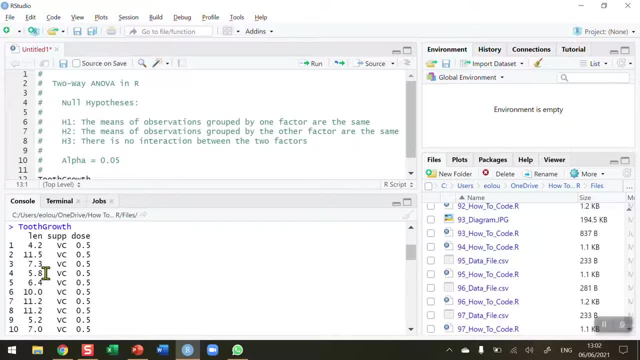 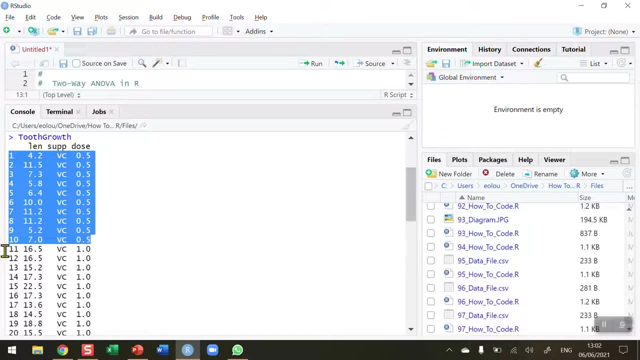 a supplement and a dose. So we can see that the first ten guinea pigs- let me just stretch this out to see it a bit more- The first ten guinea pigs are being given vitamin C and a dose of 0.5.. The second ten- 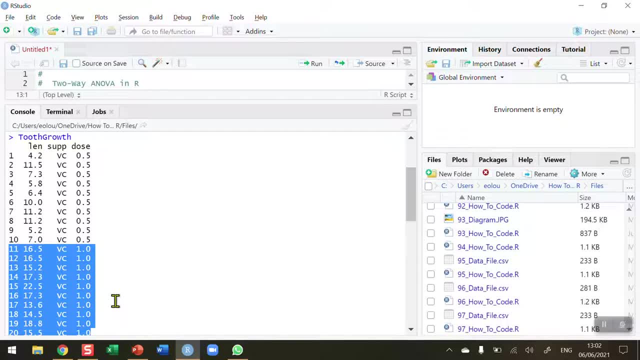 are being given a dose of vitamin C and a dose of 0.9 vitamin C, and so on, And from nine thirty one on, we move, and then we see that the second supplement is orange juice- orange juice. so we have two supplements and three different doses. to explain. 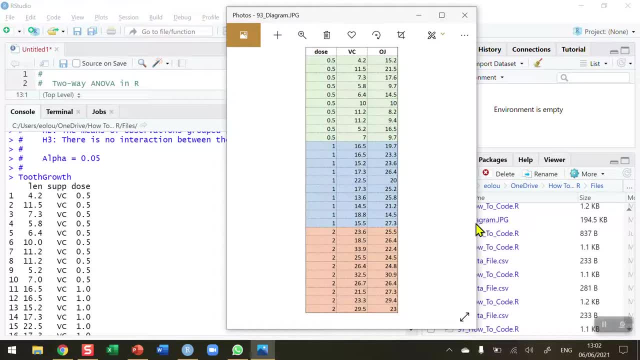 this a little bit better. I've drawn it up in a diagram on. this is an Excel spreadsheet with the same data on it. now we can see here that we've got three separate doses of 0.5: one and two. we've got the tooth growths then for the 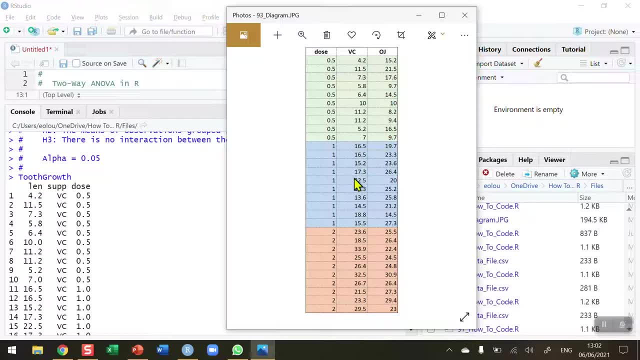 vitamin C and for the orange juice. so which are we going to look and see? is there a difference between the supplements which are vitamin C and orange juice? and we're also going to look to see if there's a difference between the three doses of 0.5, one and 2.0. and then, more importantly, we want to 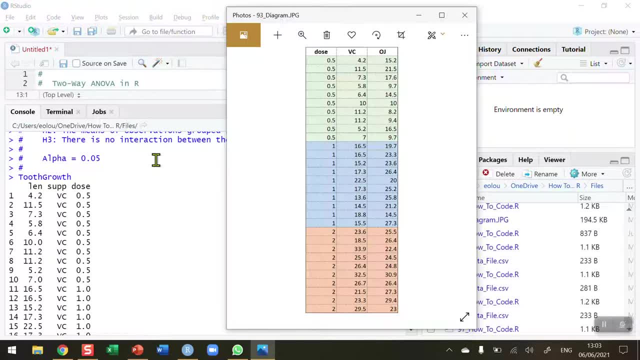 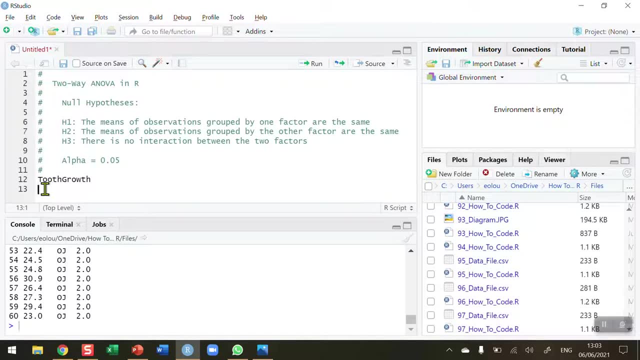 see if there's an interaction between the dose and the type of supplement. so let's go back to our code and the first thing I want to do is I want to visualize and my data. so I'm going to do this using the plot function: the plot. 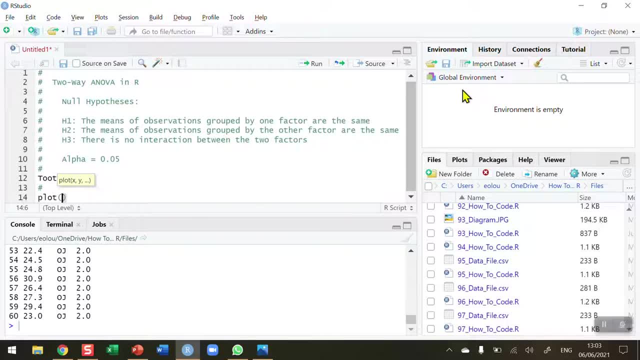 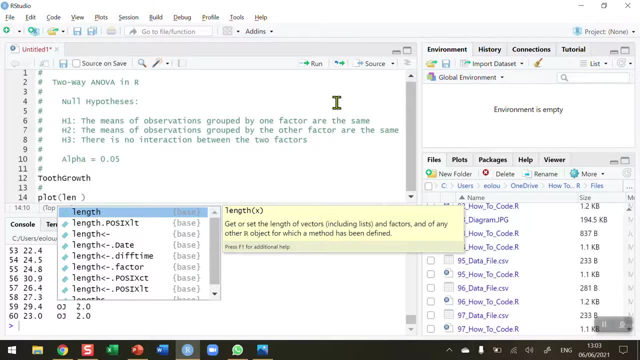 function I'm going to use is we need to add- this is a similar to what I'm going to do with the two ANOVA, so it's important that we follow along here. so Len is the length variable in the data set. so, and then I'm going to use the tilde symbol, which, in the Windows, 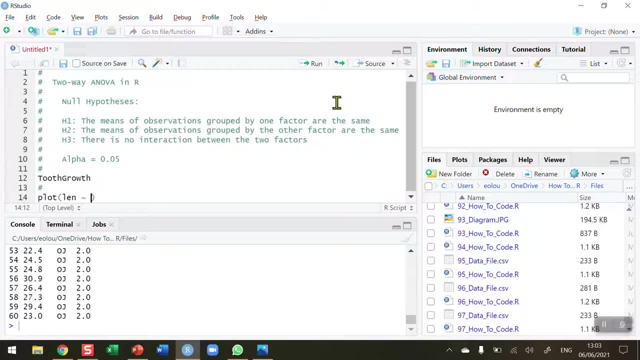 keyboard is above the hashtag key and then I'm going to the two factors, then our supplement plus factor and in brackets, dose, then a comma after that and I also need to tell or what the data set is. data set is equal to two squared taken enter there. so this, hopefully now should show me your 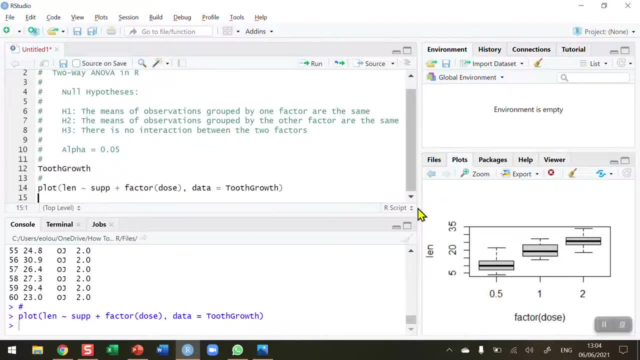 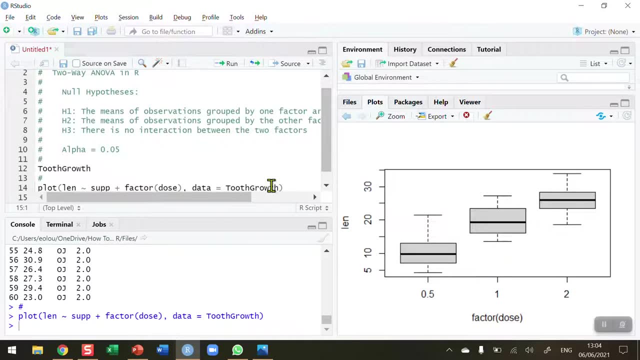 plots. let's run this line of code so we can see if I make my plot area a little bit bigger. okay, so this is the box talk here for the factor of dose, and we can see that visually. it looks as though there are differences between the three. doses in this case here. so we'd expect to find that the standard is low, so this can be calculated as positive as nine. for this case we'd expect to find sentence and no as positive as a minute number. but the cumлохница will not be- were much lower. the number is lower. so this is one thing that is not true. so it τους with our formula. and then the pros and cons. 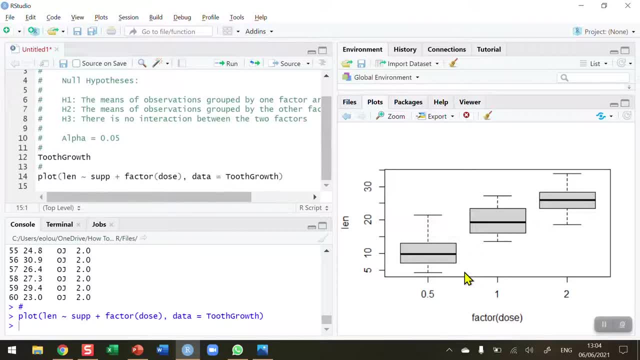 a difference using a two-way ANOVA. so just doing this for the dose factor and we get a similar result if we do it for the supplement factor. so we can see that the means the dose of two is much higher than the dose of one, which in turn is much higher than the dose of 0.0, and we do see. 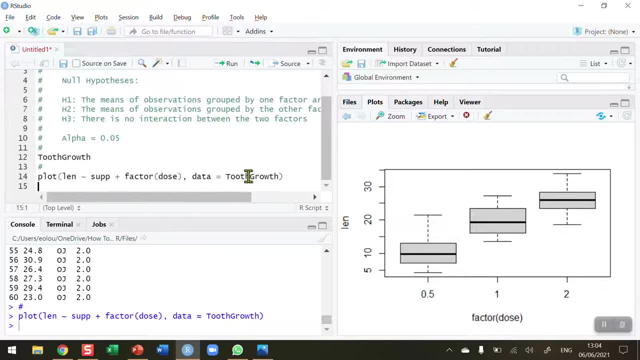 there's a little bit of overlap between one and two, but visually I would expect to find a difference between the doses. so let's now move on and perform our two-way ANOVA. and the way I would do this, I'm just going to use a temporary variable called two ANOVA, just to I can call this anything I want. 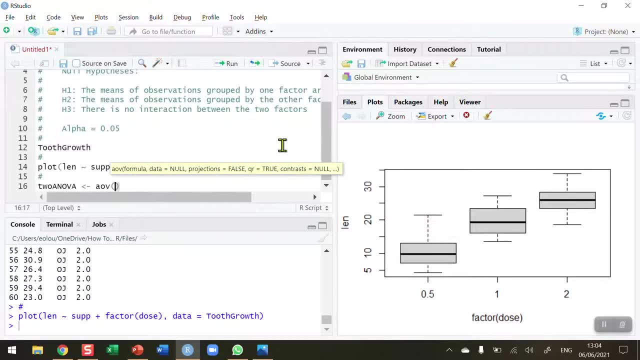 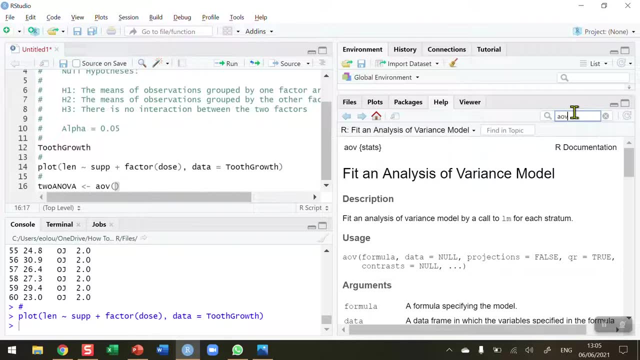 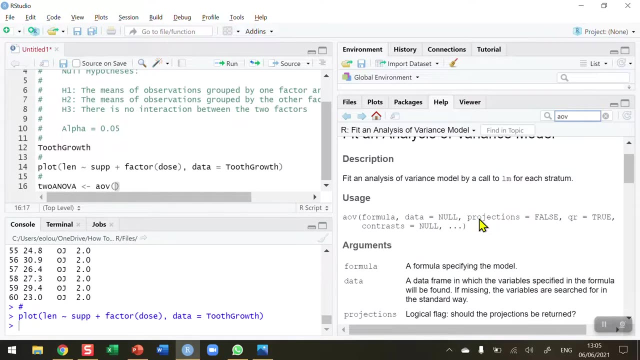 and I'm going to use the AOV function to do that now. if you haven't used the AOV function before, do it to check out the help screen type in the AOV name and it will give you a description of this formula, of this function, with some arguments and parameters and some details about the function. 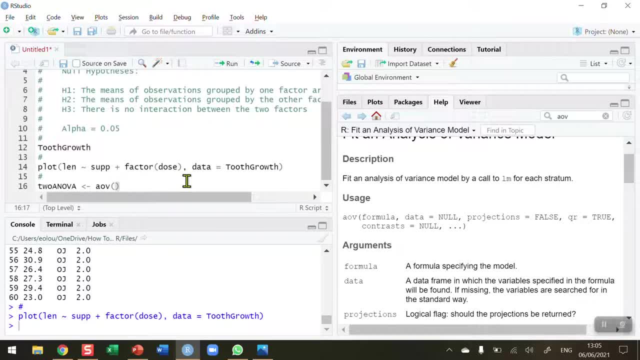 if you haven't used it before, always a good idea to look, look it up now. the piece of code I'm going to put here is is similar- not the same, but similar to what I've done for the plot. so, once again, its length is one factor, or is the measurement that we are, that we are checking? 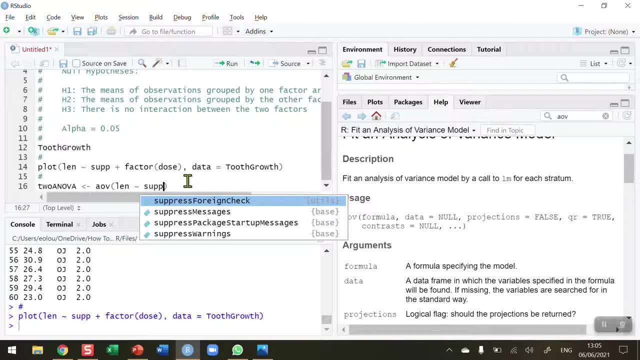 out here and supplement SUP multiplied this time. in the previous, for the box plot it was plus sign, but here we need a multiplication symbol. the asterisk factor is dose. again a comma after that and, as before, indicate what the data set at. data is equal to tooth growth. 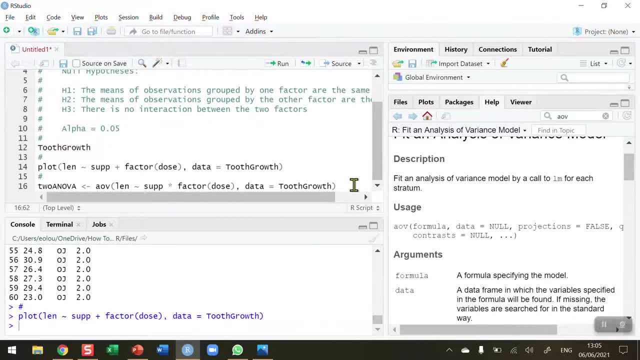 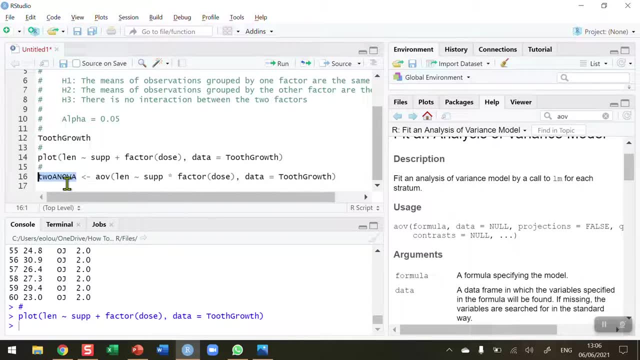 now let me take a quick look at this. I'm going to use the AOV function to store in the vector to ANOVA. my length is the is. that is the measure that we are looking for. I want to compare it in the supplement factor and the dose factor and we're taking the data from the to growth data set. 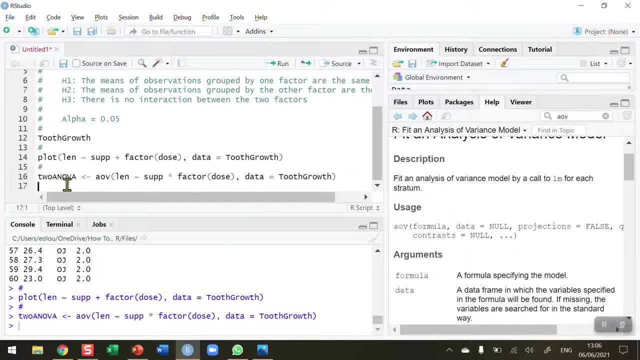 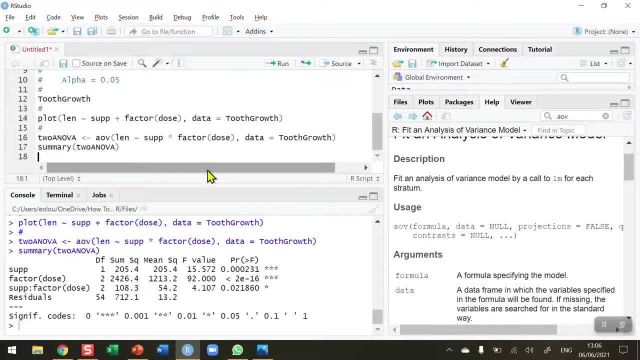 so let's run that and then when I need to use the summary function then to summarize, display my 2a table, so I'm going to use my vector that I just created here. so let's run this and we can see in the console that we get. we get the output in the format of an ANOVA table. now there's a lot of. 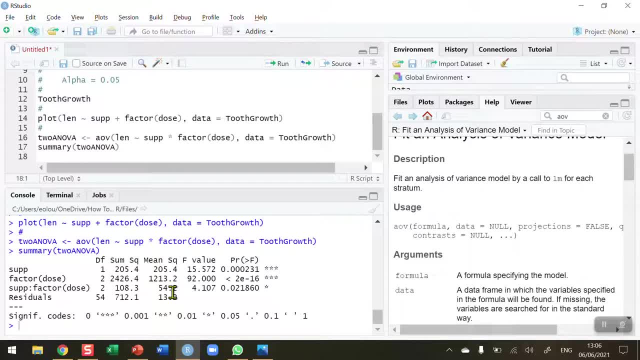 information in here, and so you should by now be aware of how what an ANOVA 2A ANOVA table looks like we can see for the supplement. let's take a look. is there a difference between the two supplements, vitamin C and orange juice? we can see that we have quite a high F value of 15.57 here. 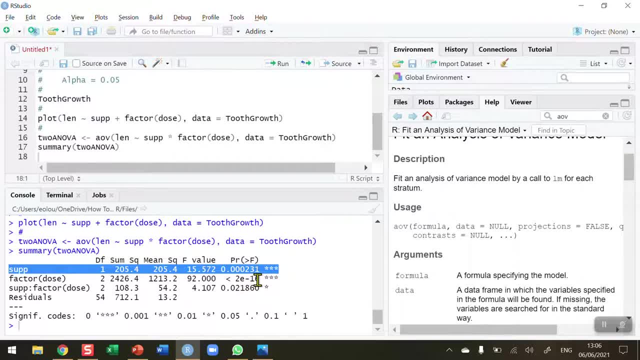 and we've got a very, very low P value. it's 0.000231 and we can see with the three asterisks that this is significant at the 0.001 level. so we have found a difference between the two supplements. there is a difference between the means of vitamin C and orange juice. moving on, 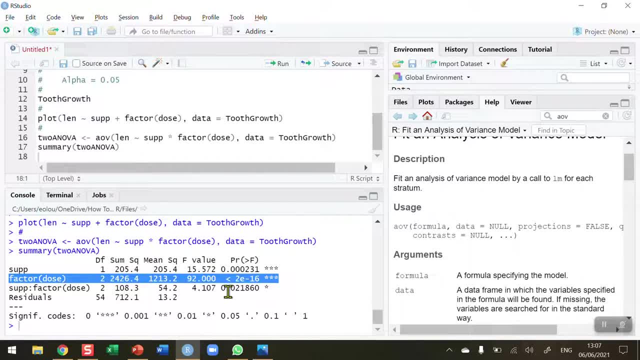 to the second line again. we've got a very high F statistic here of 92.00. we've got a tiny P value and we've got a very high F statistic here of 92.00. we've got a tiny P value and we've got a. 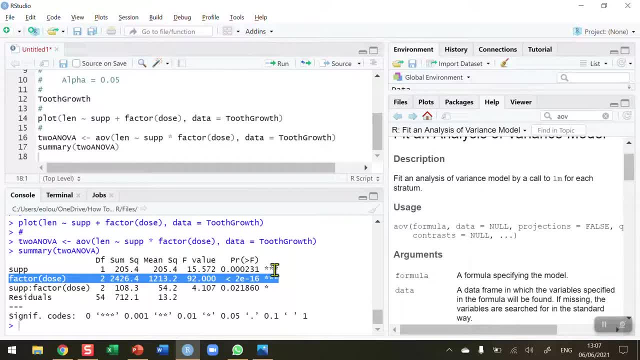 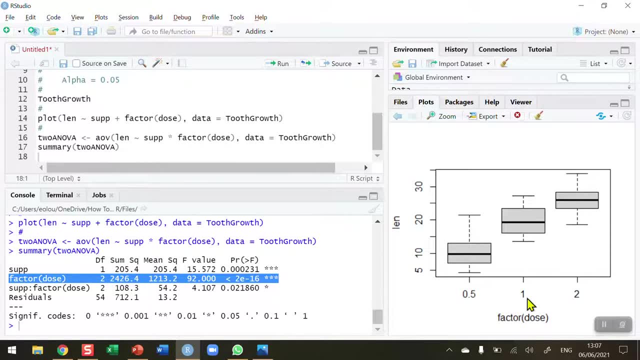 value. it's less than 2, 10 to the power of minus 16, so that's a really tiny P value and this is also a big, significant difference as well. when we look back on the plot, we can see the factors presented here, that there are differences between them, and we've now shown that there is a 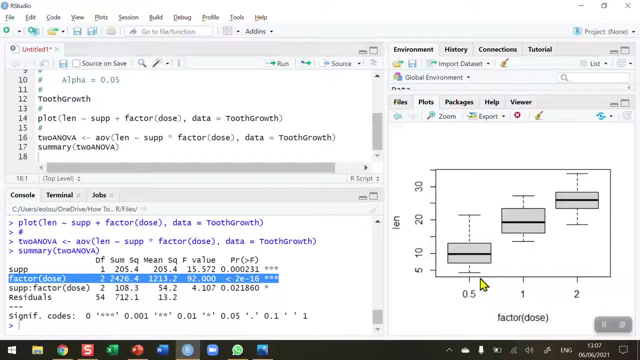 significant difference between the three factors at a P value less than 0.001. and then, finally, then the interaction with the one that we're main, one that we're looking for. we can see we've got a F value of 0.001 and we've got a much smaller F value- F statistic here of 4.107, and we've got a 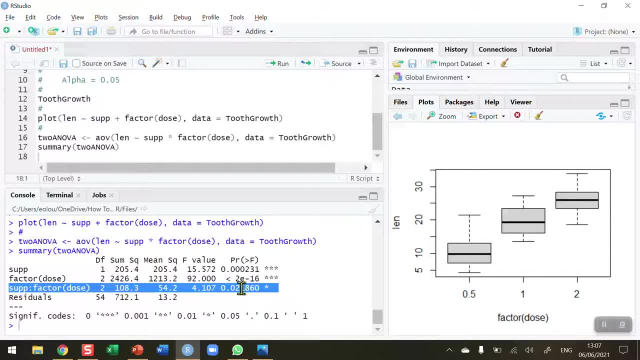 F value of 0.001 and we've got a much smaller F statistic here of 4.107 and we've got a. we have got a P value of 0.0218. so at the alpha value that we set initially, we cannot reject a. 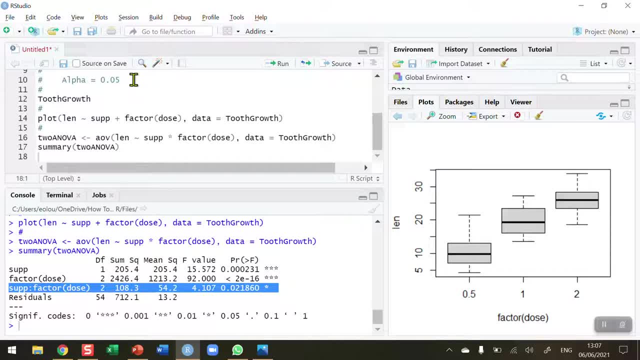 null hypothesis here, because we can reject a null hypothesis at that value. sorry, 0.02 is less than 0.05, of course. so we have found we can reject the statement that there's no interaction between the two factors in favor of the alternative hypothesis is that there is an interaction between the two. 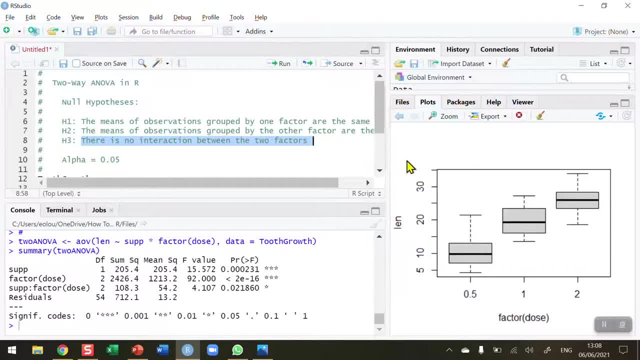 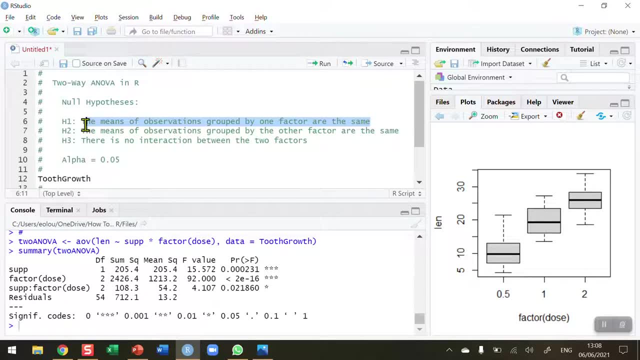 factors. so, looking at these three hypotheses again, we in fact have a P value of 0.0218 and we've got a. we reject all three hypotheses. so we have found a difference between the first factor, which is the supplement, we have found a difference between the second factor, which is the dose, and we have found